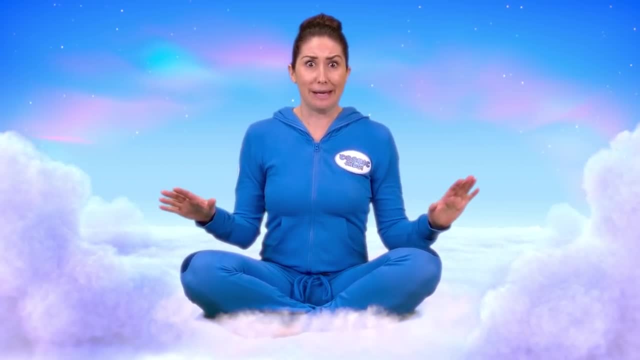 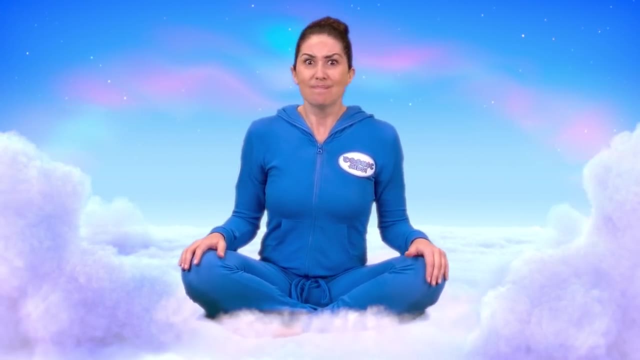 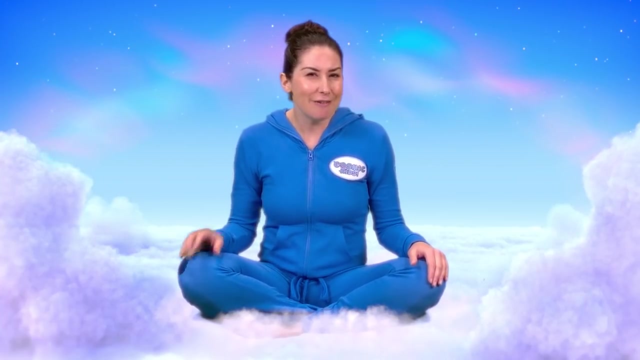 something, Anything: Balancing on one leg, Reading, Reading, reading a new big word, lying or sitting still or solving a puzzle, As you try. often, quite soon after you start, a very little but powerful thought pops into your mind. 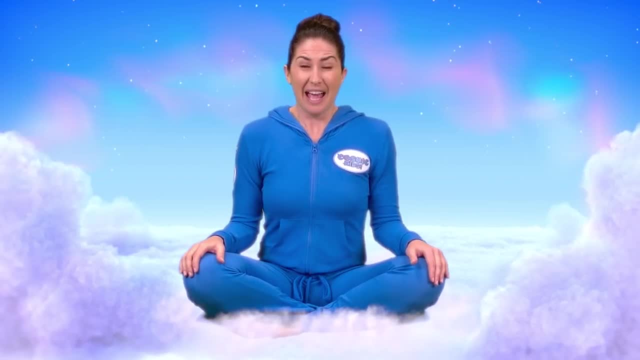 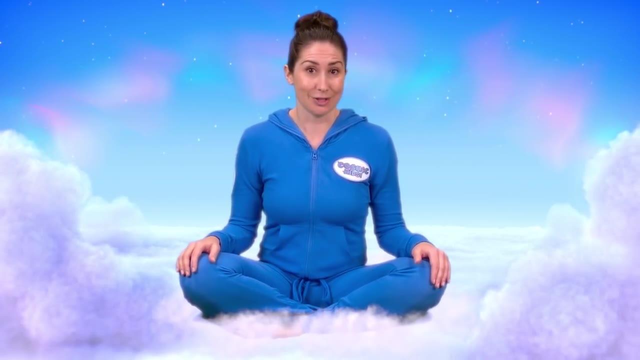 I can't do this, And we all get this when we try something for the first time. And the best way to make the I can't thought go away is to think: oh yes, I can. The I can't thought is like a little naughty monster who will suddenly jump in. 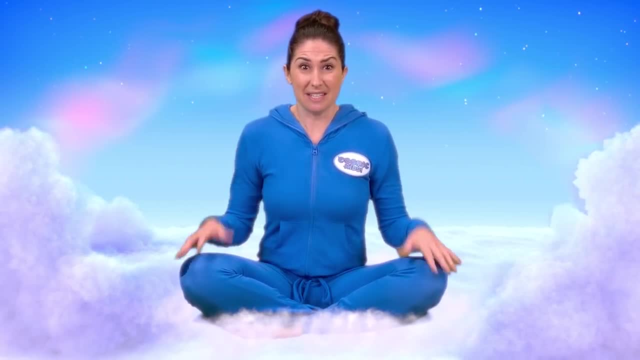 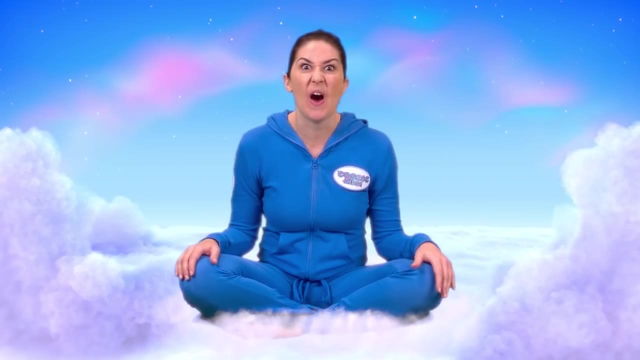 and make you feel all weak and annoyed and maybe even frustrated with what you are doing. All he ever says is: oh no, you can't, Oh no, you can't. When the I can't monster appears and all these hard feelings start, 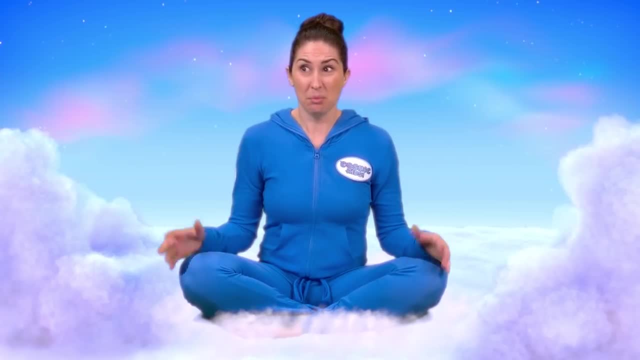 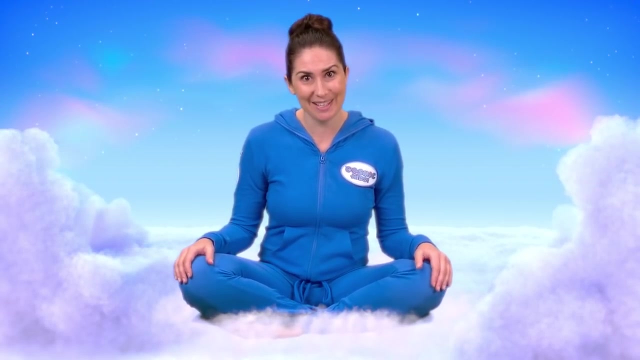 it becomes even harder to do what you are doing. More thoughts appear: I'll never be able to do this. This is a waste of time, I'm bad at this, And each of these thoughts make it harder to do what you are trying to do. 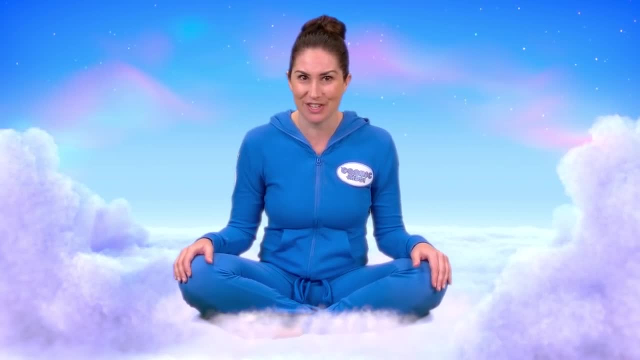 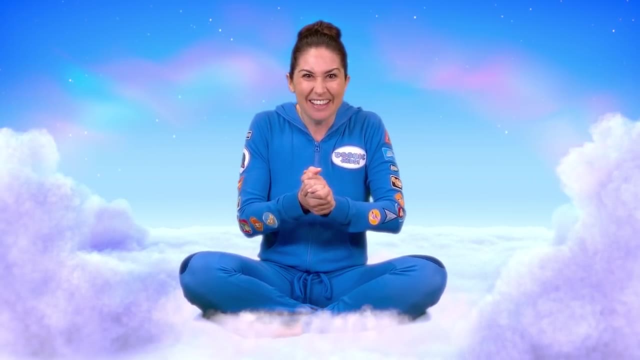 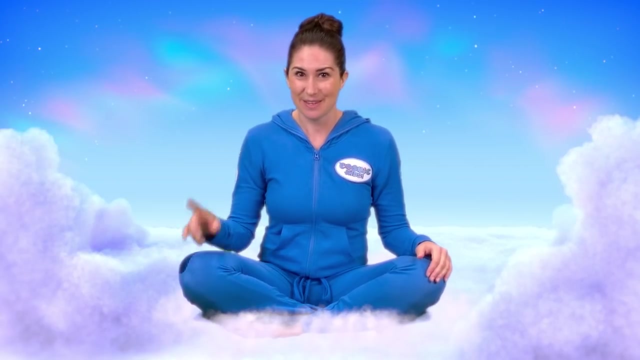 The I can't monster is always ready to jump out when you do something new, Something for the first time. He's rubbing his hands together just waiting for things to get difficult, Which they always are when you first try something, So be ready for him. 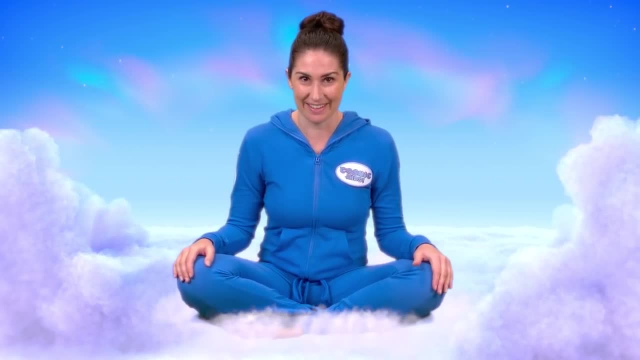 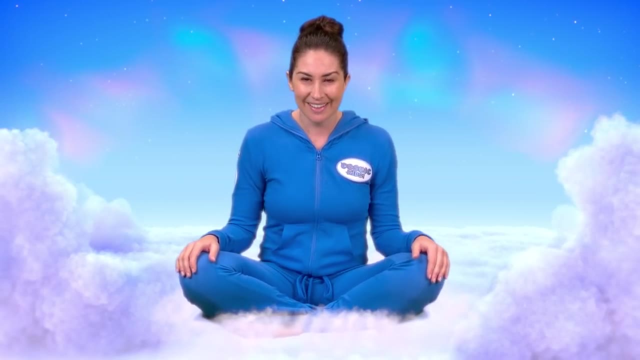 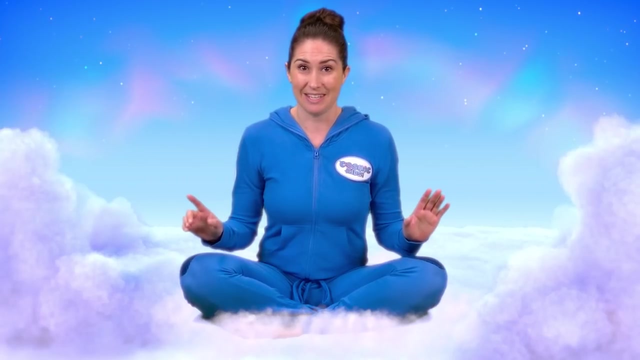 The next time you are trying to do something, see if you can spot the very second. the I can't monster pops into your head. When you spot it, smile to yourself. Smile to yourself Because just by spotting it you will be able to squash it. 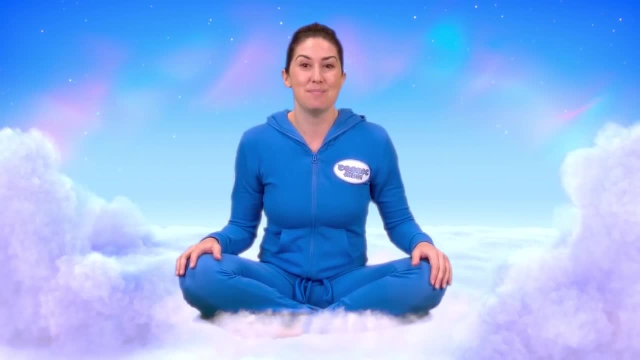 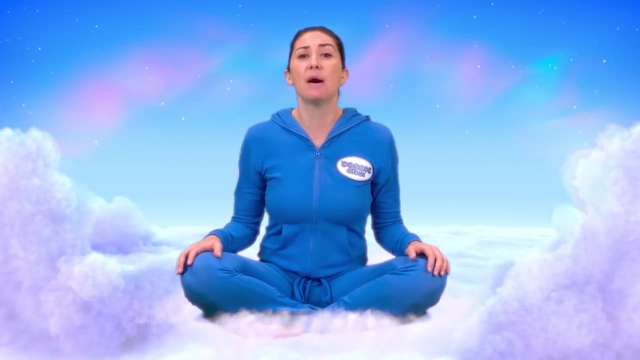 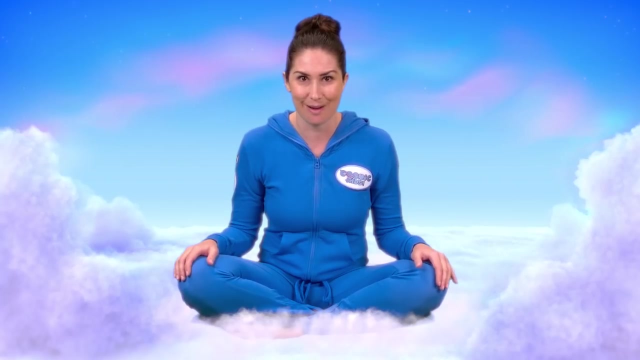 And the thing that really squishes him is when you say back to him: oh yes, I can. Then he disappears into a puff of smoke. The more you practice saying oh yes, I can, the weaker he becomes And you get stronger and stronger.